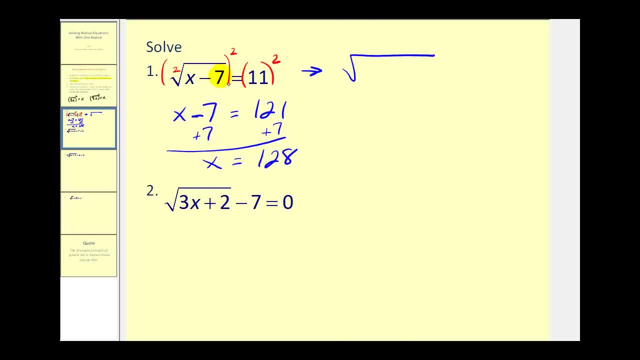 Does the square root of one hundred twenty-eight minus seven, that's one hundred twenty-one, equal eleven, And it does so. it checks On number two. we need to add seven to both sides to isolate the square root before we square both sides. 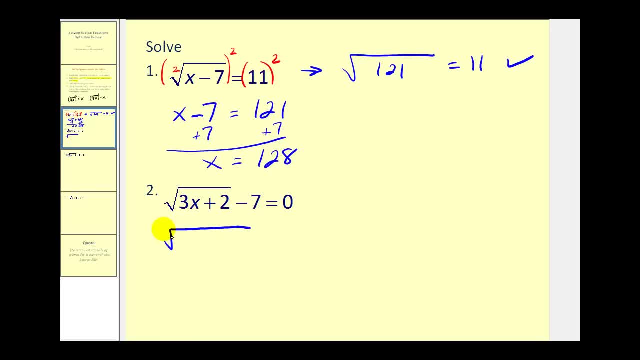 So if we add seven to both sides, we would have the square root of three x plus two equals positive seven. I always like to put the index in here just to remind me that I'm going to square both sides. So the square root of three x plus two squared will be: 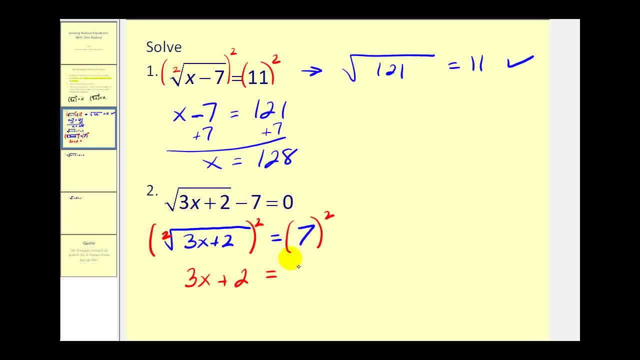 three x plus two equals seven. squared, that's forty-nine Subtract two on both sides, that would give us three x equals forty-seven. Dividing by three, we have x equals forty-seven-thirds. Now you might think that's going to be hard to check. 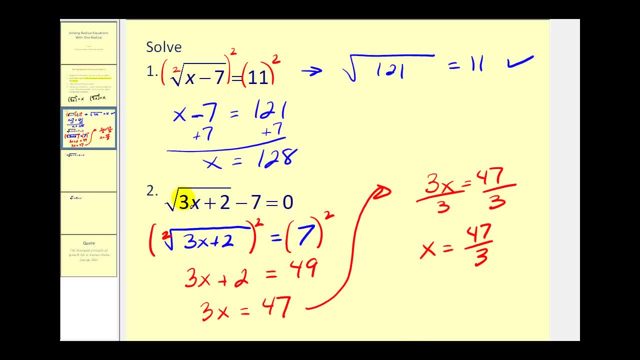 but look what happens when you sub in forty-seven over three and then you multiply by three. Those threes are going to simplify out. so this would become forty-seven plus two, which is forty-nine. The square root of forty-nine would be seven minus seven equals zero. 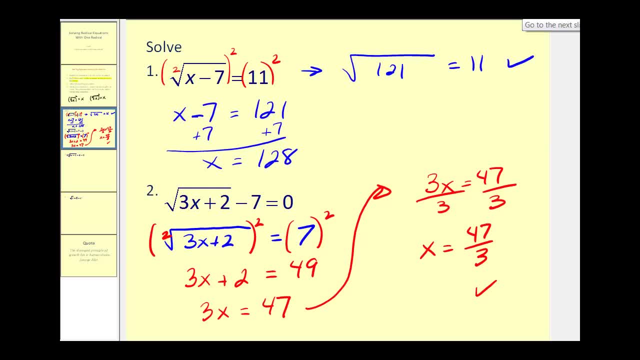 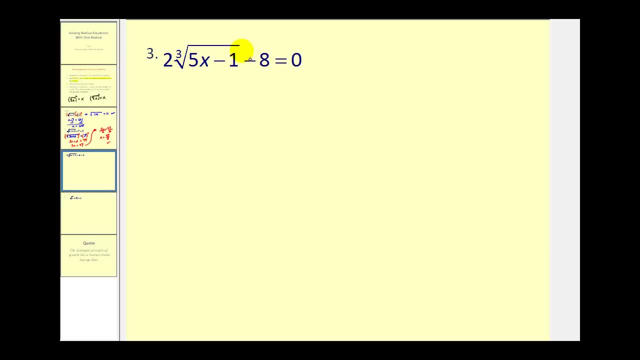 So this checks as well. Let's go ahead and try a couple more Again. the first step here is to isolate the radical, or in this case the cube root, So we should add eight to both sides. Next, this two is attached by multiplication, so we should: 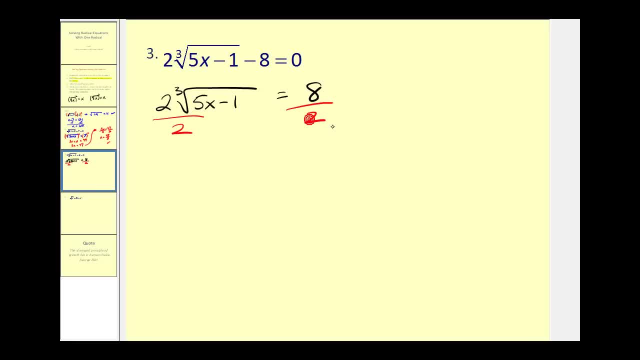 divide both sides of the equation by two, So we have the cube root of five x minus one must equal four. Now our index is three, so we'll raise both sides of the equation to the power of three, The cube root of five x minus one cubed. 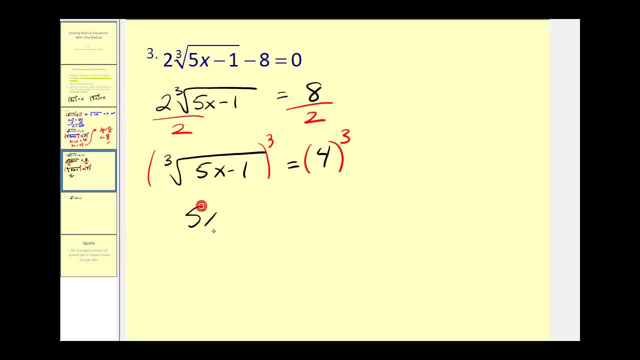 will just be: five x minus one equals four to the third power would be sixty-four, So we'll add one to both sides. That would become sixty-five divided by five. X equals sixty-five divided by five would be thirteen, And we can go ahead and check. 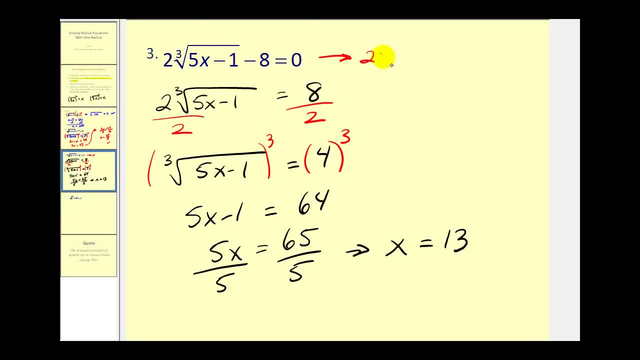 this as well. Two times the square root of five times thirteen would be sixty-five minus one. That would be sixty-four minus eight equals zero, And again this is the cube root. So the cube root of sixty-four would be four. So two times four is 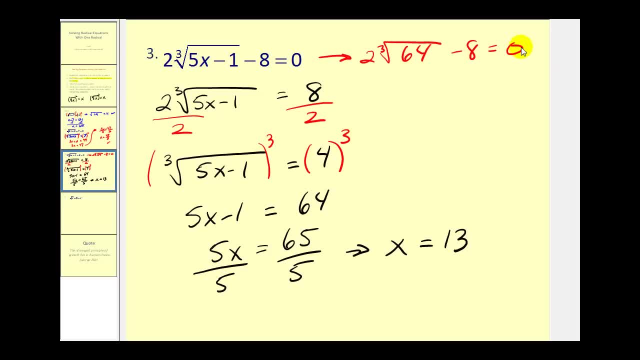 eight minus eight is zero. It checks. And let's take a look at one more. Remember, before we start, we must isolate the square root. So we're going to subtract six on both sides, So we'll have the square root of x. 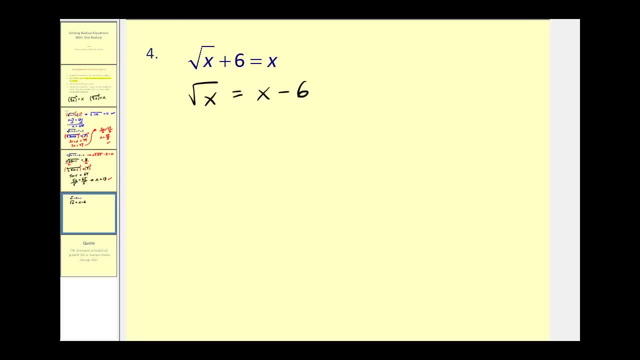 equals x minus six. It's a square root, so we'll square both sides of the equation. We're not squaring each term, we're squaring both sides. So on the left, we're going to have x. That's good. On the right, we actually have to. 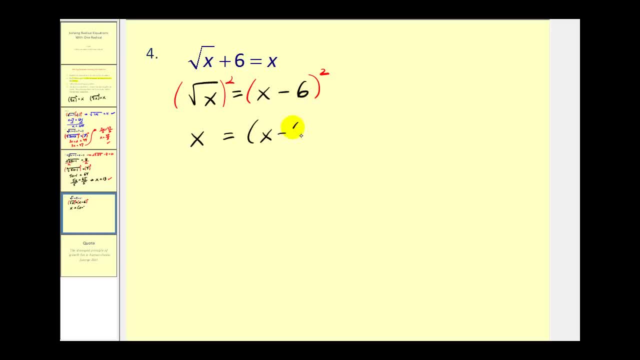 multiply this out: X minus six times x minus six. Remember you can't just square x and square six. So we have x equals. this would be x squared Minus six, x minus six, x, That's minus twelve, x Plus thirty-six. Okay, we have a quadratic equation now, So we're going to set it equal to zero and see if we can factor it. 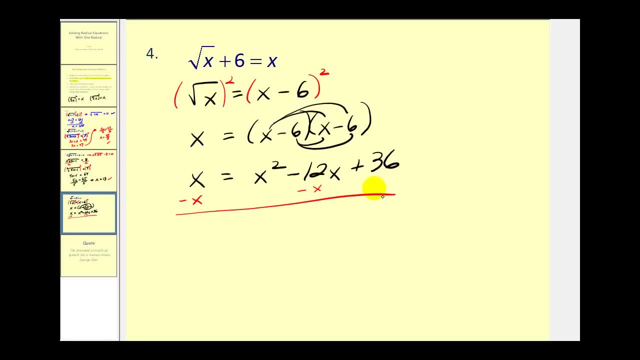 So if we subtract x on both sides, we're going to have zero equals x squared minus thirteen, x plus thirty-six. I believe this is factorable Factors of x squared x- x. Are there factors of thirty-six That add to negative thirteen? And there are. 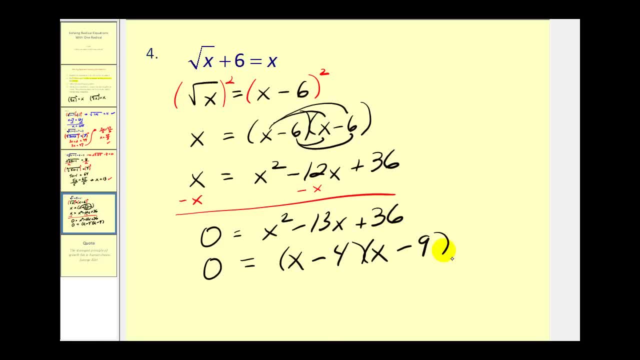 Negative four and negative nine. Okay, so it looks like we may have two solutions: Either x equals four or x equals nine. But let's go ahead and check these to make sure. Let's check x equals four first. We'd have the square root of four. 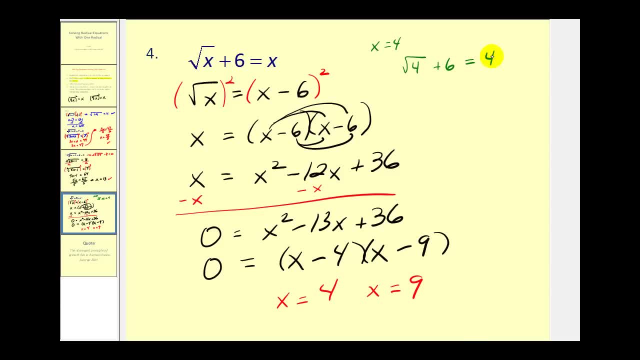 plus six equals four. Well, this doesn't work. That would be: two plus six equals four. That's not true, Which means this is one of those extraneous solutions, So we cannot include that as a solution. Let's go ahead and check. x equals nine.